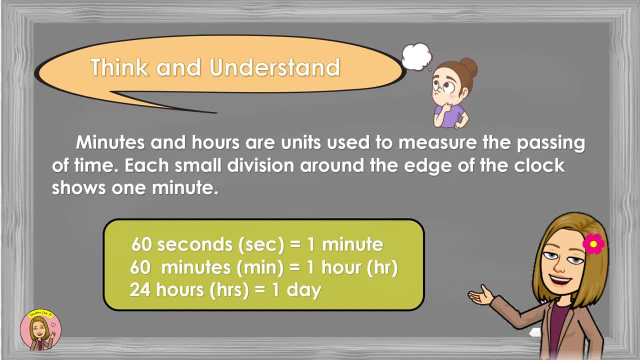 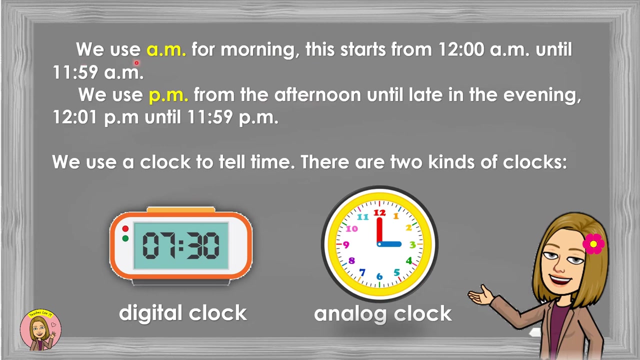 Minutes and hours are units used to measure the passing of time. Each small division around the edge of the clock shows one minute. Sixty seconds is one minute And sixty minutes is one hour. Twenty-four hours is one game. Less than6 minutes is a game. 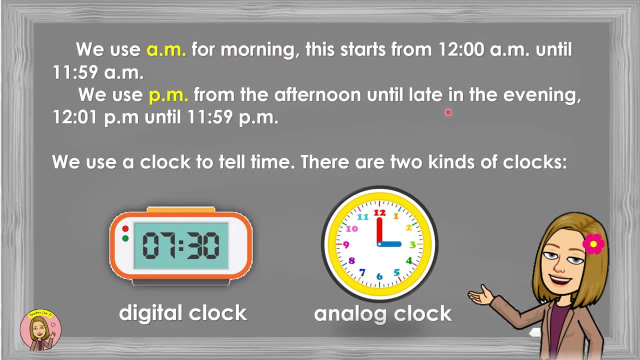 We use em for morning. this starts from 12 am until 11: 59 jego. We use eM from the afternoon until late in the evening. this starts from 12 am until 1159 em. We use eM from the afternoon until late in the evening. 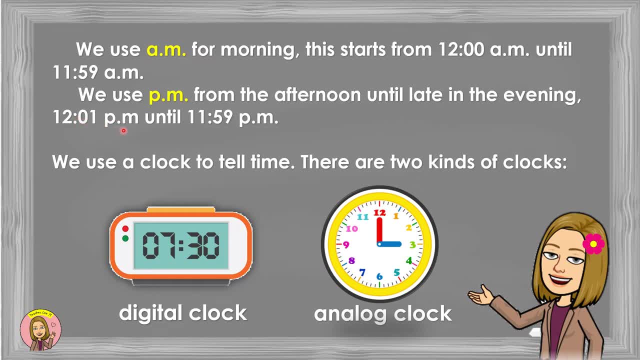 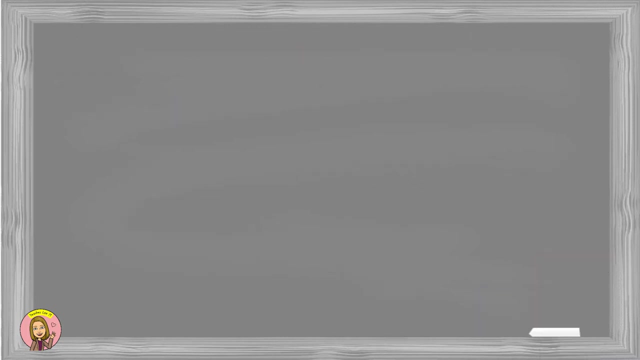 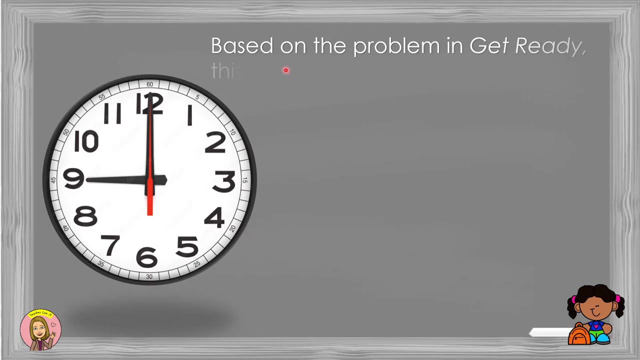 12.01 pm until 11.59 pm. We use a clock to tell time. There are two kinds of clocks: Digital clock and analog clock. Based on the problem in Get Ready, this clock shows 9 o'clock. 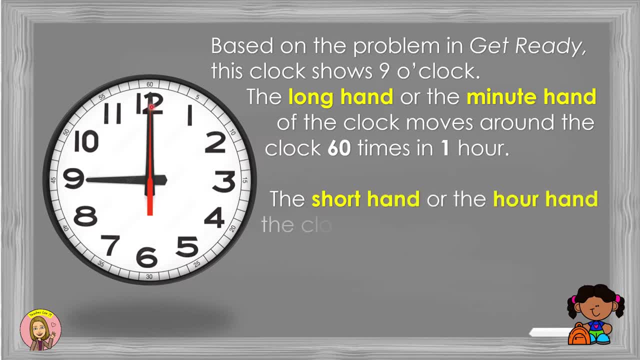 The long hand, or the minute hand of the clock moves around the clock 60 times in one hour. The short hand or the hour hand the clock has moved past 8 towards the 9.. We can use Keep Counting by Fives to read the clock. 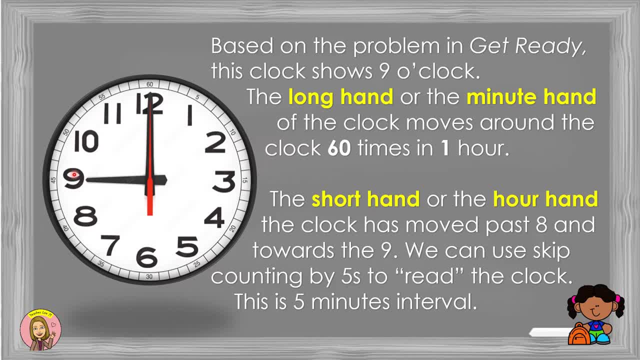 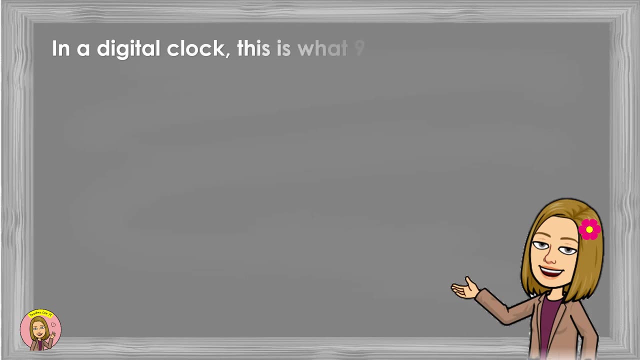 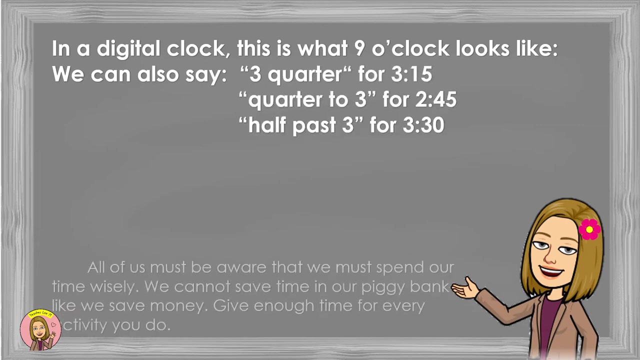 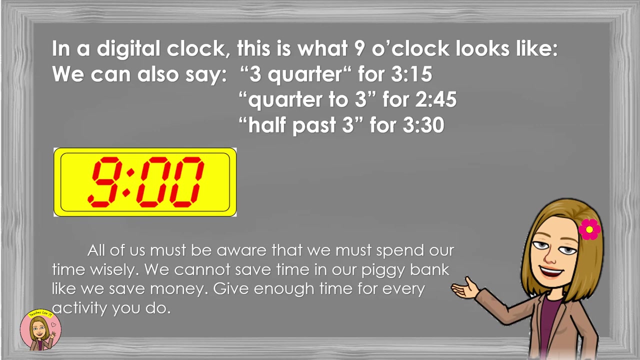 This is 5 minutes interval In a digital clock. this is what 9 o'clock looks like. We can also say 3, quarter for 350,, quarter to 3,, 4 to 45, and half past 3.. 4, 3, 30.. all of us must be aware that we must spend our time wisely. we cannot save. 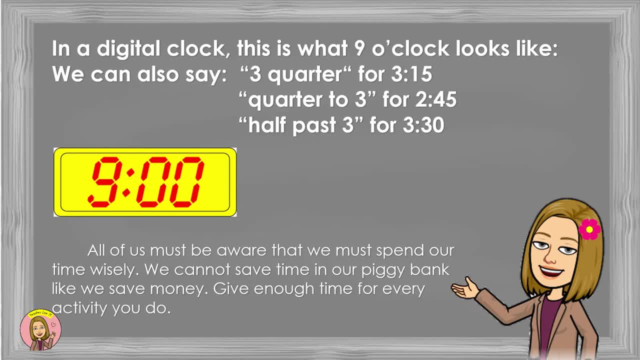 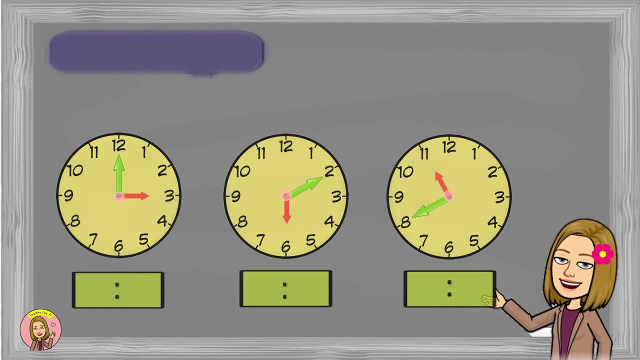 time in our kiki bank, like we save money. give enough time for every activity you do. what time is it? write the time that each clock shows. i will give you 10 seconds to answer. time's up. it's three o'clock six ten. it's 11: 40.. great job. 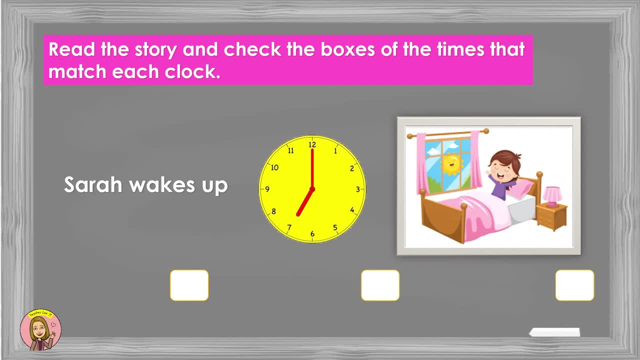 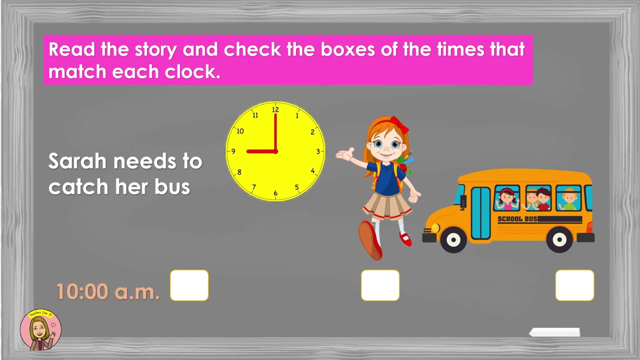 read the story and check the maxes of the times that match each clock. sara wakes up. what time? sara wakes up. at 7: 00 am. sara needs to catch her best. what time sara needs to catch her best? what time? what time?